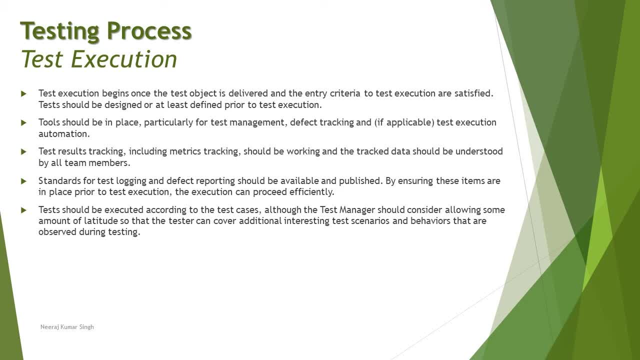 only begin because you can have internal entry criterias to determine that have you finished what you were supposed to finish and what you were supposed to finish and what you were supposed to finish before you can get into the execution and can definitely have an entry criteria for that, as 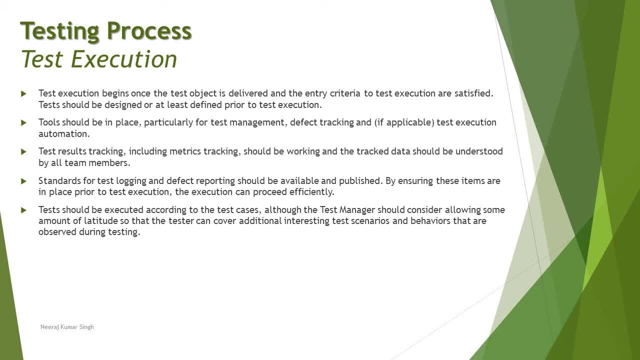 well and once it is satisfied, you can definitely step into your execution process. On the other side, of course, the tool and the environment must be well established and validated, evaluated before you can enter into the execution phase, and a lot of other tools which are basically to track the 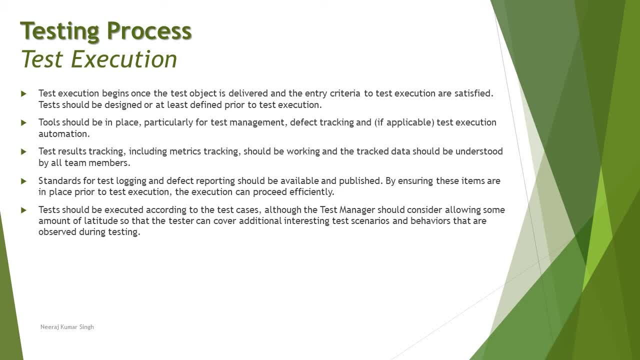 progress and manage your defects, because during the execution you definitely welcome a lot of defects, So everything must be well executed and you can definitely get into the execution phase to make sure that everything is well executed and well placed within the environment in order to make use of it. So these are a lot of things. So test results tracking is another important thing, because 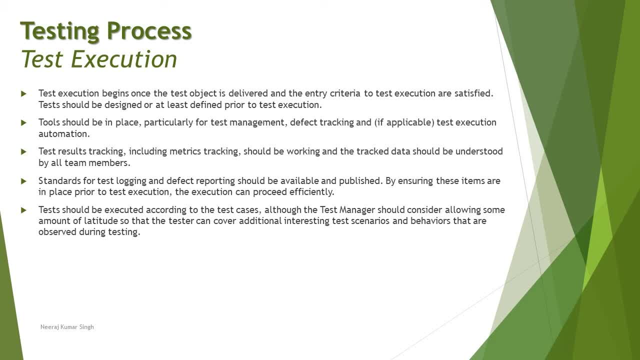 ongoing monitoring of any activities will be taken care of with these kind of tracking process and any kind of deviation if observed, the test manager has to take the necessary control actions to overcome those deviation. Now this deviation can have examples like talking about a blocker or not, a non-availability of any kind of test data or any such thing which might be interrupting. 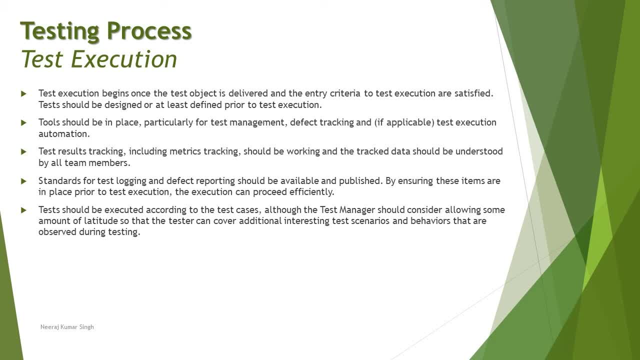 your execution has to be taken care and necessarily attended with the control action. Even if you talk about the logging of the outcomes of the testing should be, well you know, captured, because you must have a tool like test management tool which generally allows you to simultaneously capture. 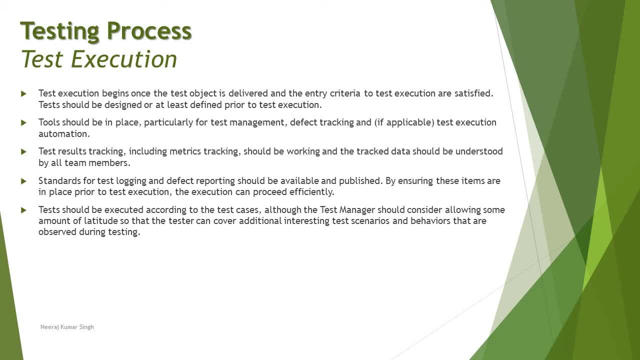 the actual results as well, based on the execution and a lot, many other factors related to the execution, For example, the screenshot, probably capturing a screenshot of the defect or maybe exceptions which you see other than the test case being executed, because at any point of time a test case can have a particular objective. but 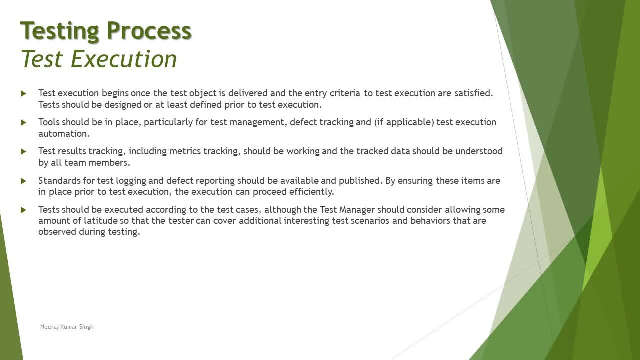 maybe your test case has passed but had certain exception, So what about that? So those things must be well captured and you should have the process and the tool available to do that job And, of course, we have created a test execution schedule as a part of the test implementation. 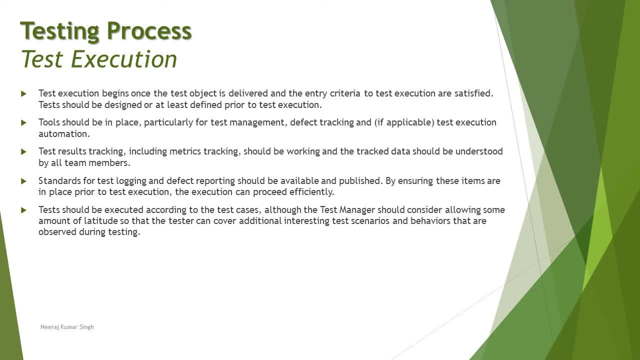 schedule. So we have created a test execution schedule as a part of the test implementation schedule. So we have created a test execution schedule as a part of the test implementation phase and we just wanted to make sure that everything is executed as per the test execution. 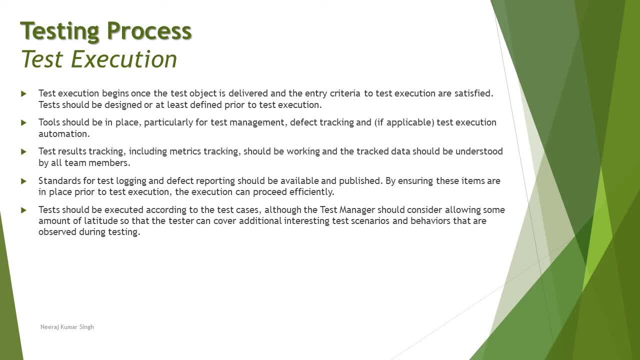 schedule. But at any point of time, if test manager realizes that there is something specific which must be accommodated in between, then reprioritization could be done as a part of the control action, depending on any kind of- you know- source stoppers or any kind of blockers which you 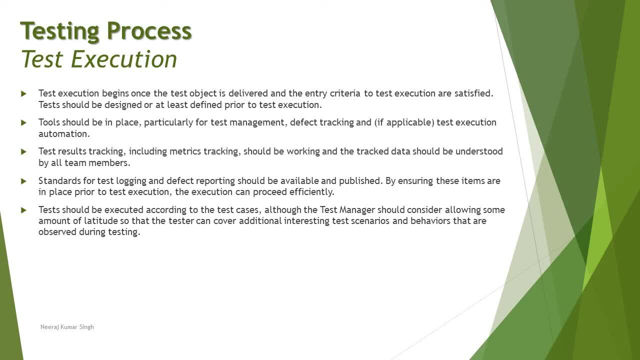 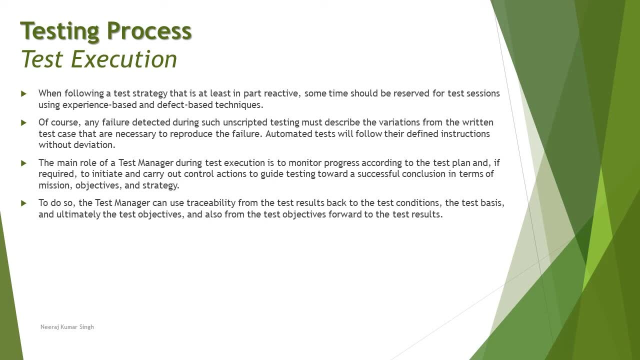 may experience as a part of your process at any point of time. Further to add, of course, when following a test strategy that is the least in part reactive, sometimes should be resolved for the test sessions using experience-based and defect-based techniques. That means you do have a lot of you know- test cases being designed or derived with. 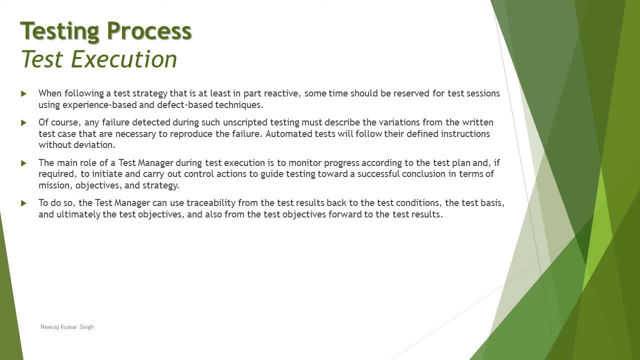 help of the formal techniques like equivalence, partition, boundary value analysis or design decision table testing, straight state transition testing, and there are a lot of things which you generally make use of in a test strategy. So that's why we have created a test execution schedule for you to make use of, So you just need to make sure that whatever you're trying to do, it must be. 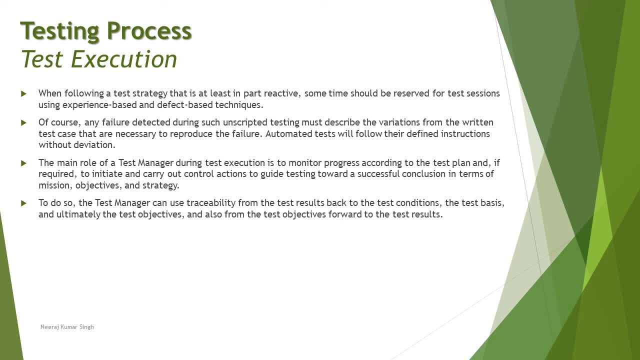 following the strategy, which you're making sure, and, as a part of the strategy, if, in case, you have experience-based techniques someplace for that, then make sure that you have enough time to run those sessions and find some different defects as well And failures. of course, the defects has to. 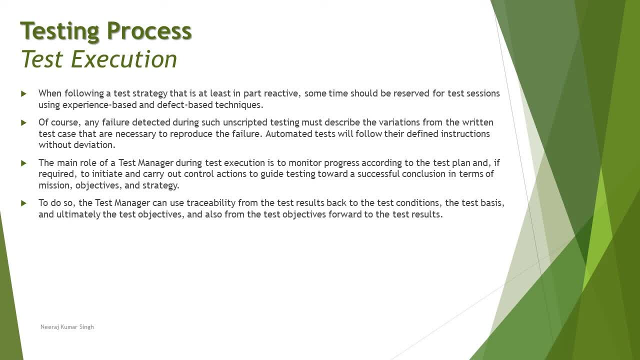 be captured. so you must definitely predetermine what template, what level of detail you must be making use of when you come to the execution process and capturing those information, with all information, what you really want to capture in order to enable another stakeholder to understand. that should be very well captured. The main role of test manager during the test. 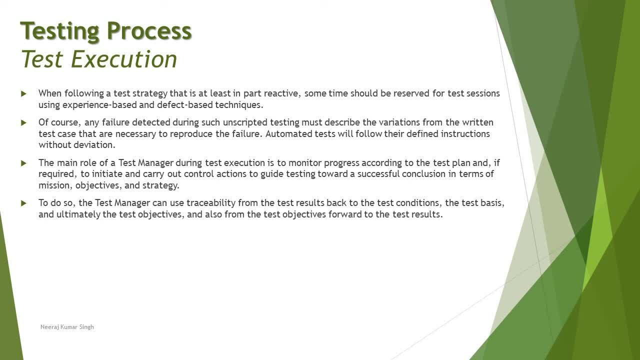 execution is to monitor the progress according to the test plan and, if required, initiate and carry out any control action to guide testing toward a successful conclusion In terms of mission objectives and strategy. to do so, the test manager can use traceability from the test result back to the test condition, the test basis and, ultimately, the test objective itself. 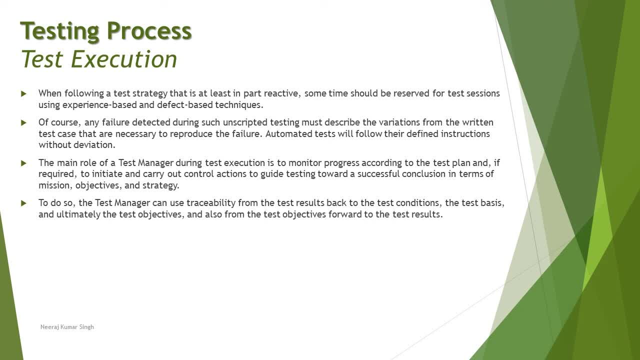 and also from the test objectives forward to the test result at any point of time. Well, this is what a lot of information which you need to be aware of being a test manager and must know the process in and out from the consideration that how exactly execution must be carried out. So, the test manager,